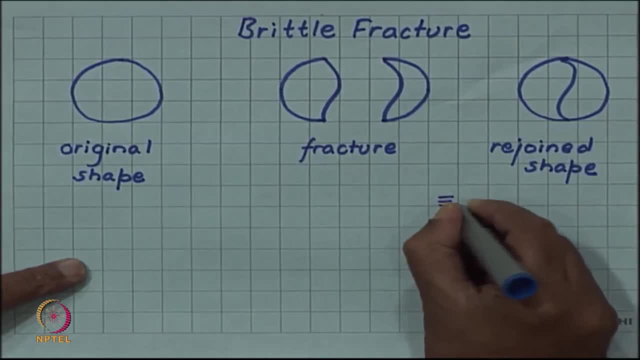 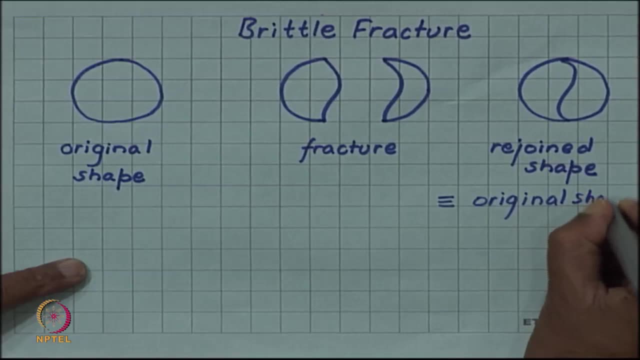 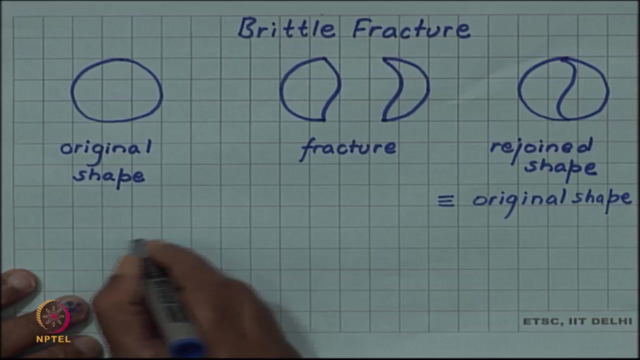 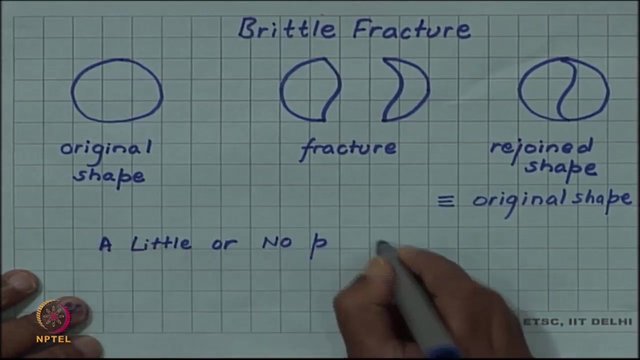 So rejoin shape is the same as original shape. All of us know that if some glass piece breaks then we can join them with some adhesive to regain the original shape. So this means that there has not been much plastic deformation before fracture, So little or no plastic deformation. 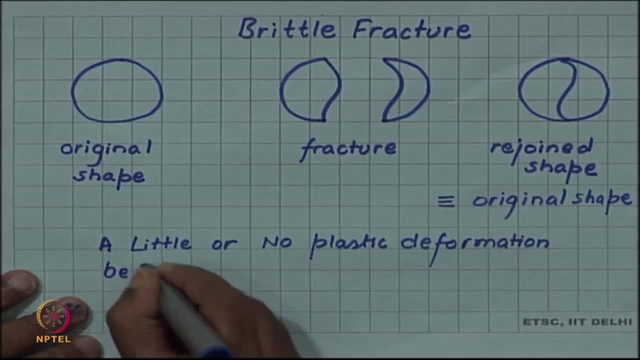 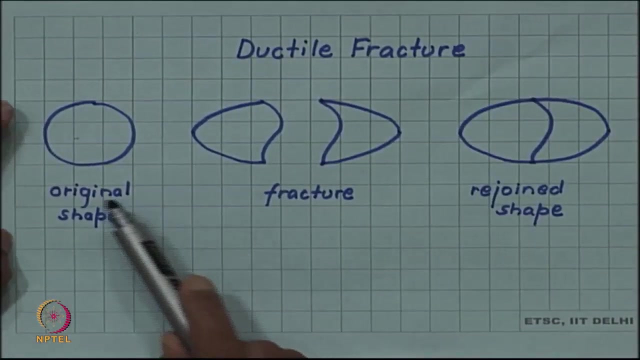 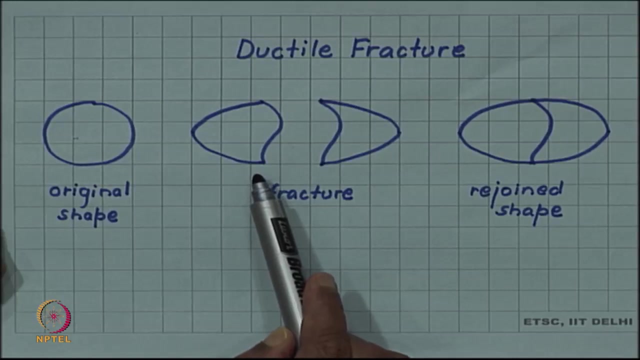 before fracture. In ductile fracture there is significant plastic deformation before fracture happens. So original shape deforms plastically before it cracks. So in this case, if we rejoin the cracked pieces, So in this case, if we rejoin the cracked pieces, 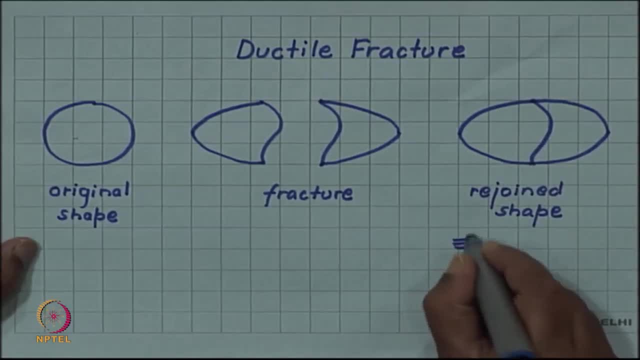 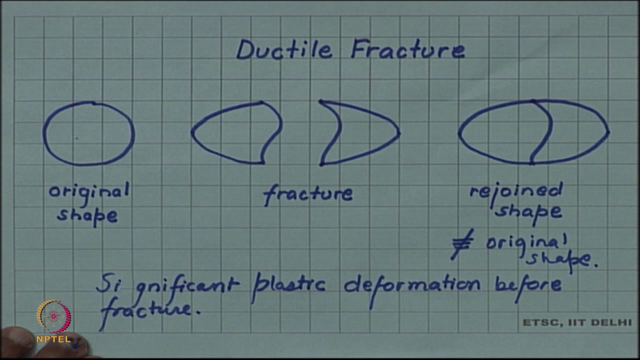 We will not recover the original shape. This is not the same as original shape. If we try to look at this, so there will be significant plastic deformation before fracture. If we try to look at this, so there will be significant plastic deformation before fracture. 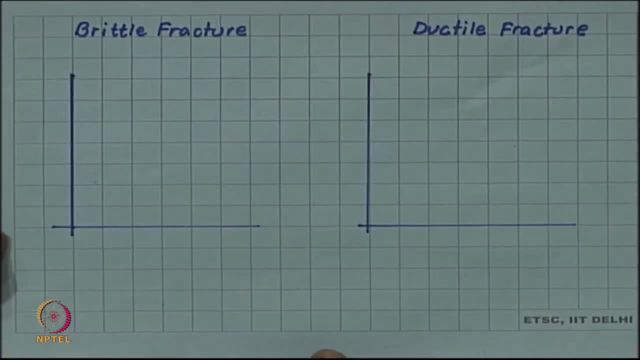 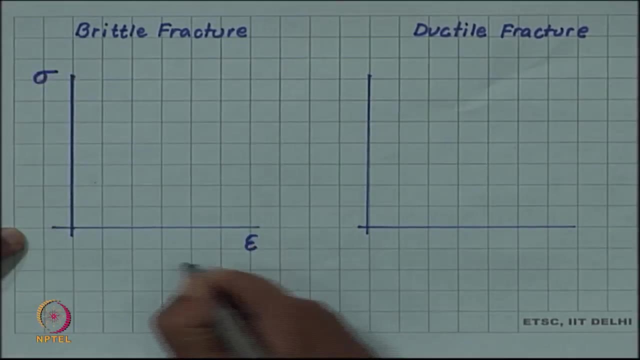 If we try to look at this, so there will be significant plastic deformation before fracture. Now, if we look at this in terms of stress and strain- stress and strain diagram- So in case of brittle fracture, actually, since there is no plastic deformation, there is no. 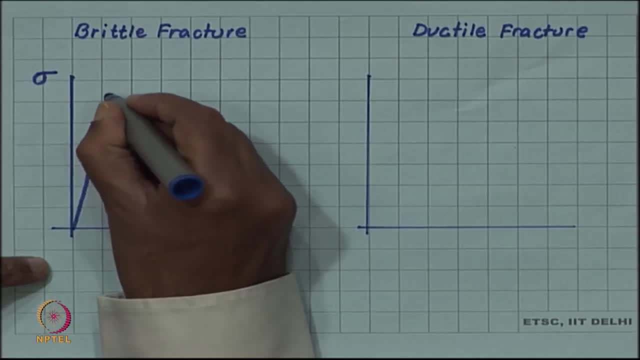 ül, But how we can re reusir it, How we can decide. if there is a fracture Now in genommen, we are talking about in conjunction- Fracture will happen in the elastic regime itself. So this is the fracture point. you 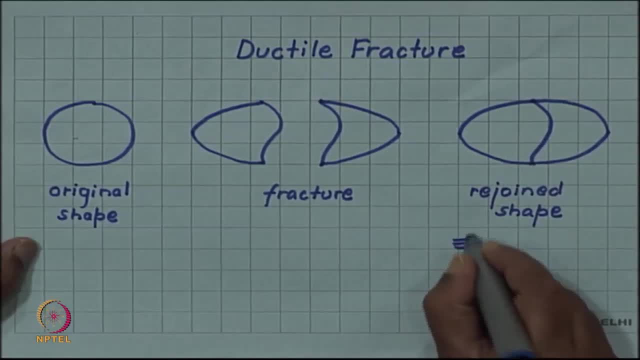 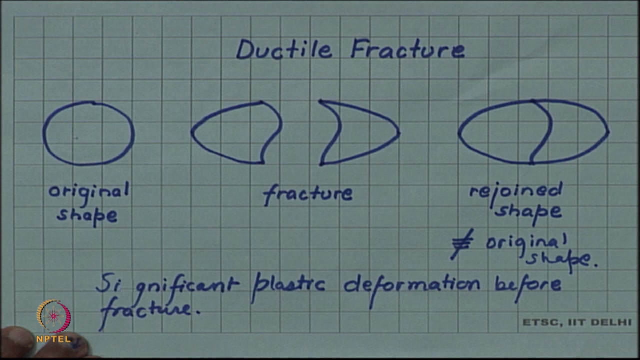 We will not recover the original shape. This is not the same as original shape. If we try to look at this, so there will be significant plastic deformation before fracture. If we try to look at this, so there will be significant plastic deformation before fracture. 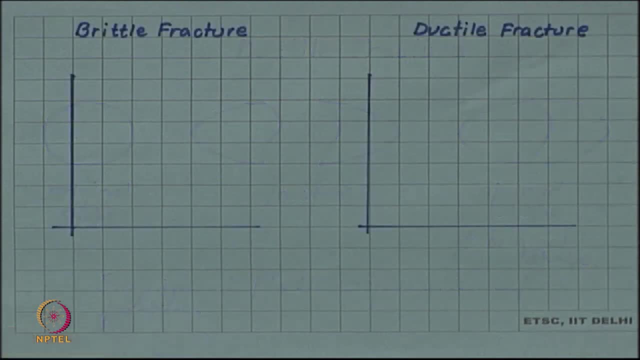 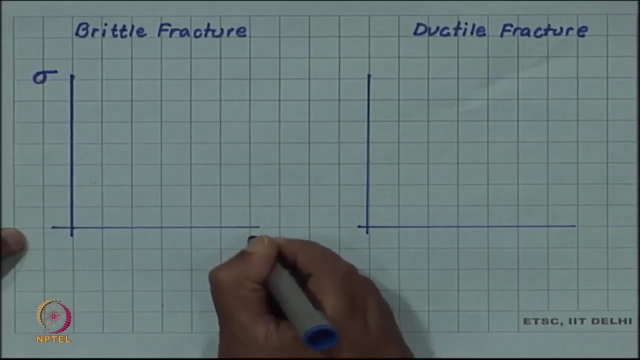 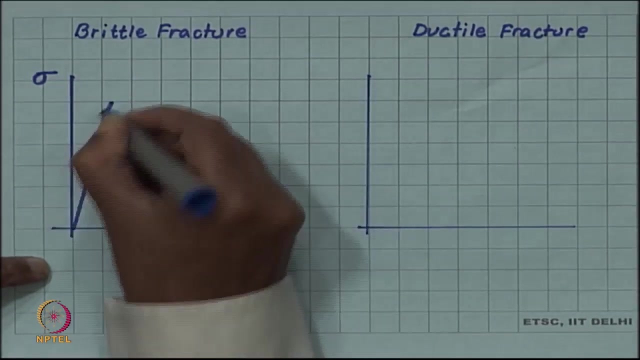 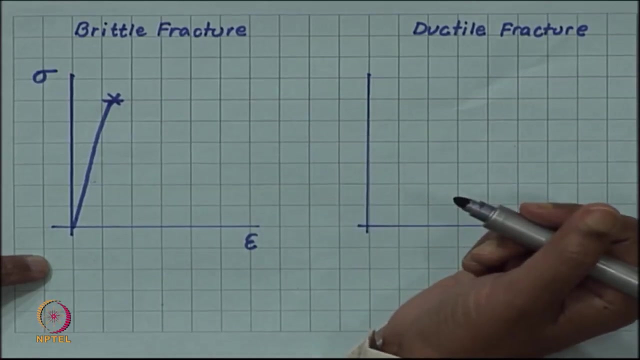 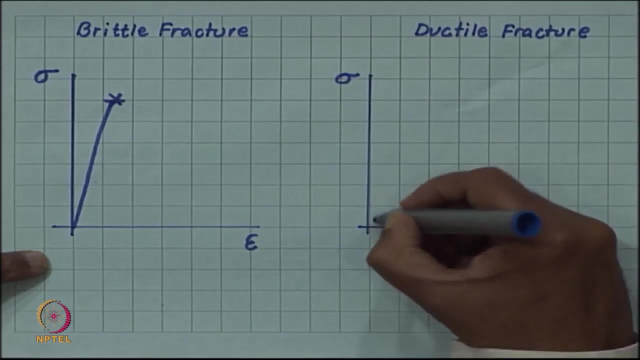 Now, if we look at this in terms of a stress and strain diagram, So in case of brittle fracture, actually, since there is no plastic deformation, Fracture will happen in the elastic regime itself. So this is the fracture point. you have a straight line elastic region, Whereas the stress strain diagram for ductile material. 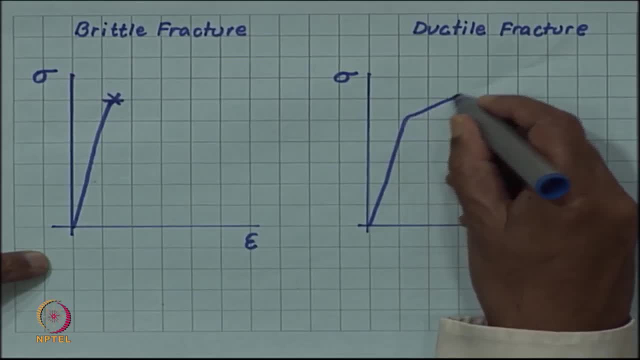 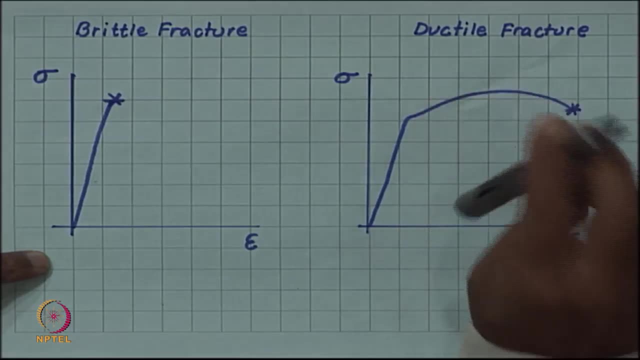 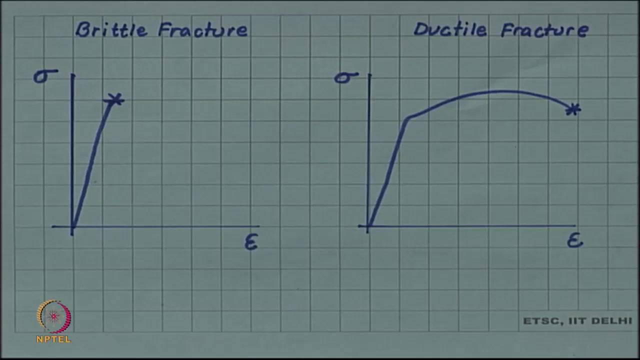 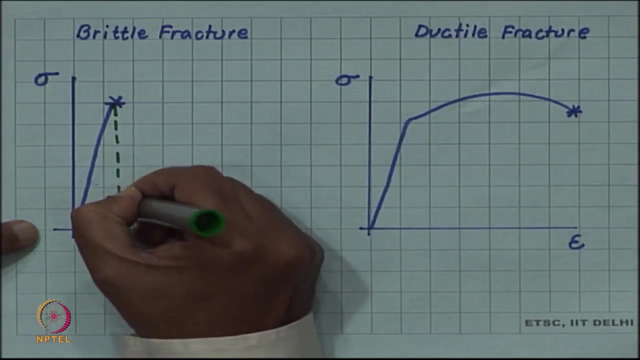 will show significant plastic deformation. So there will be lot of deformation before it fractures. So you can see that in terms of the two fracture behave differently in terms of the energy absorbed. You know that the energy absorbed in up to the point of 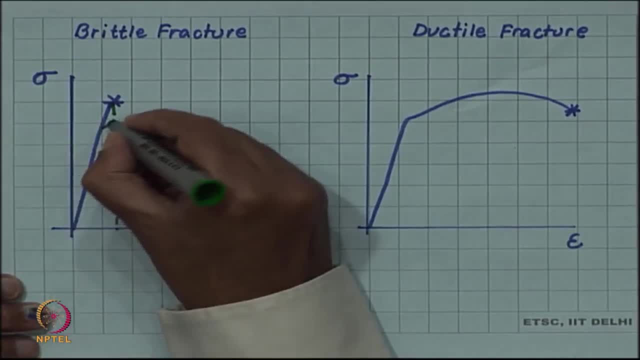 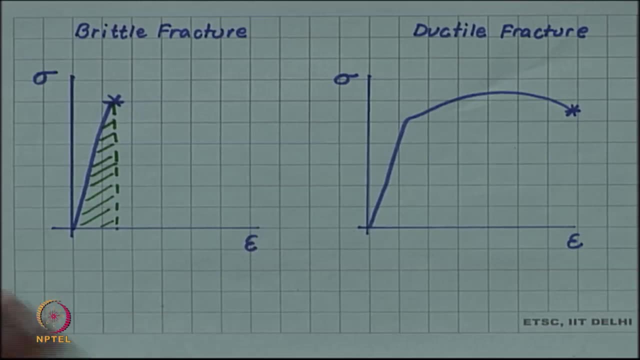 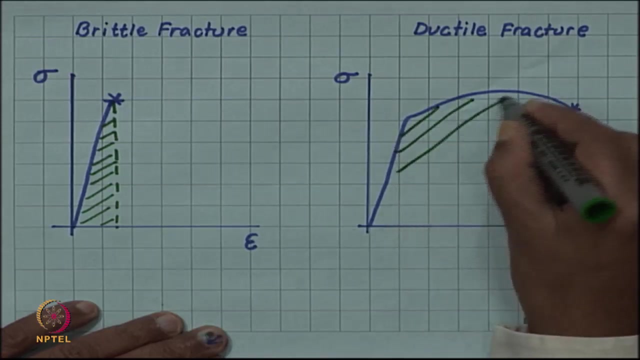 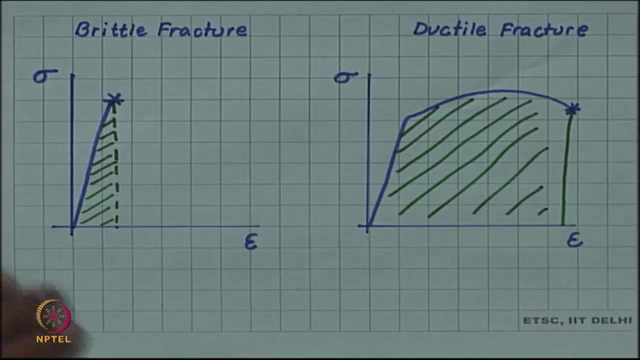 fracture in a stress strain diagram is given by the area under the curve. So since in brittle fracture, So this area will be much less compared to that in the ductile fracture. So the energy absorbed in brittle fracture is very less, Whereas energy absorbed in ductile fracture. 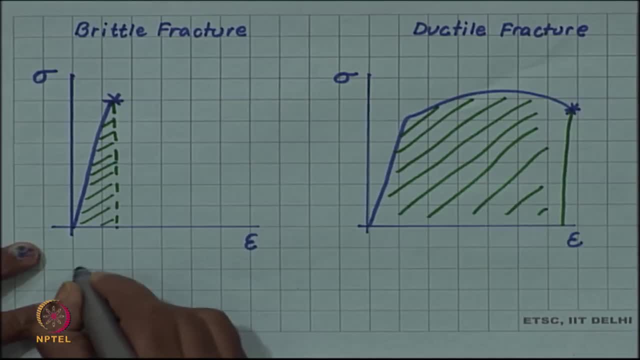 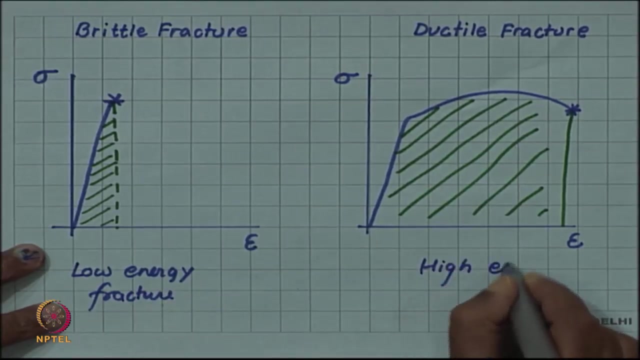 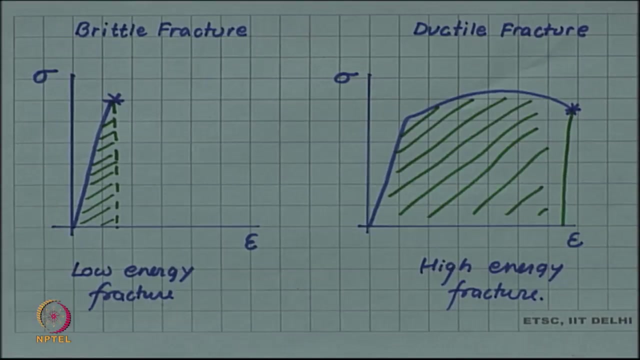 is much more, So it is a low energy, So we can call it: it is a low energy fracture and this is a high energy fracture. . . . .